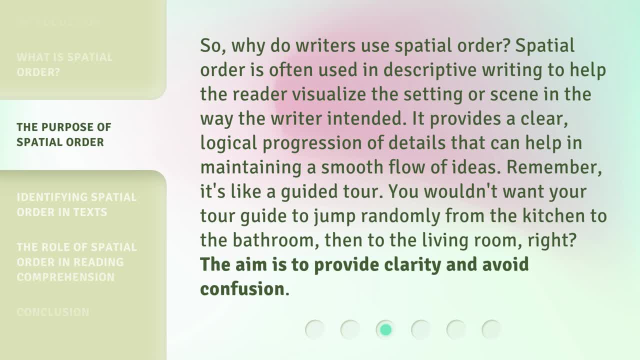 So why do writers use spatial order? Spatial order is often used in descriptive writing to help the reader visualize the setting or scene in the way the writer intended. It provides a clear, logical and logical understanding of the text. Spatial order is a method of organizing.